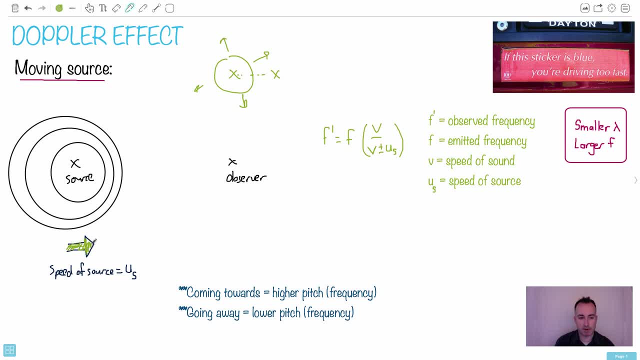 this source is going this way right here. You can see that by the squishness of these waves here that have been sent out. It's a little bit hard to draw this, because this is a dynamic situation that's actually happening and moving, whereas here I'm trying to just draw like a snapshot of what's going on. But 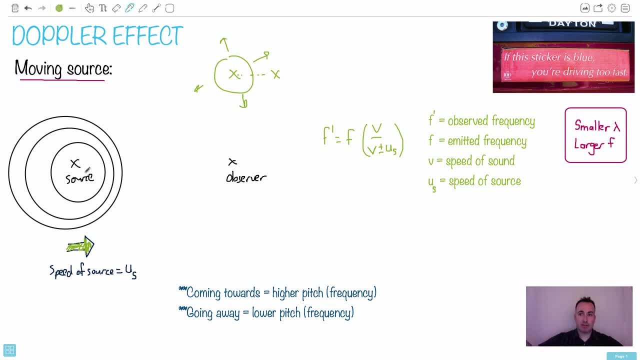 basically, what happens is as you emit these, you know these, these pulses of sound, for example. whatever these are, they're going. if you were not moving, they would just go out radially outwards. You'd see these. nice, you know. 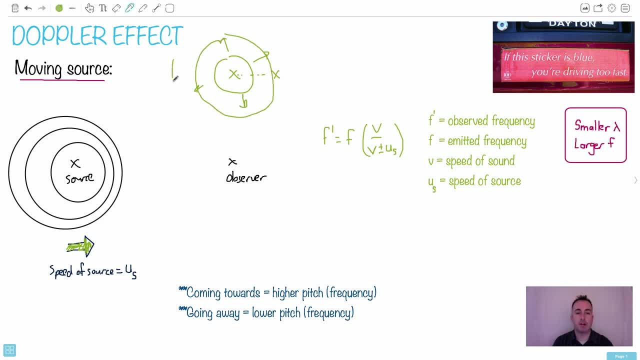 imagine, like, let's say, I set on another one, there'd be another one, and then there'd be another one, Like there'd be nice, even spaces. The problem is they're not doing this. I'm not staying still, I'm moving. So you can see as I'm moving, I'm 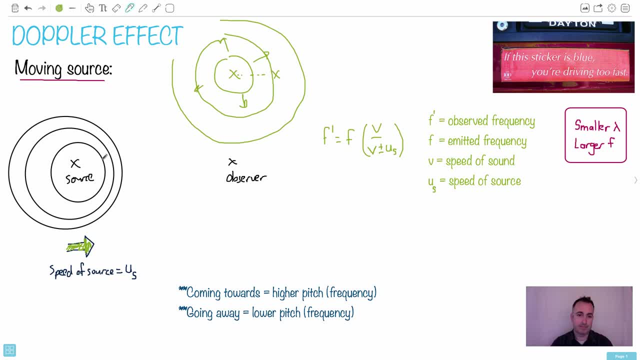 sort of squishing them as I send out another one and another one. So just this is what's going on here. I just wanted to maybe try to show this, just so it makes it maybe a little bit more sense here. So what I'm gonna do then is attempt well. 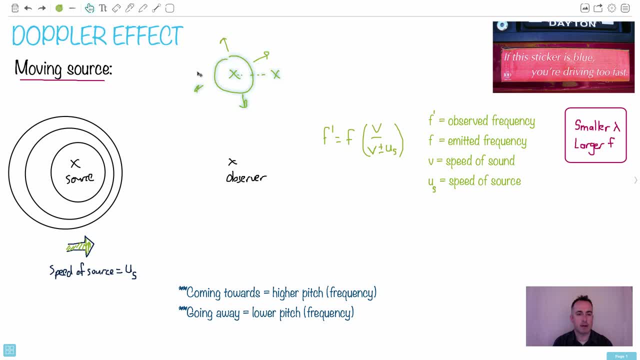 let's just see here, can I grab these and delete them? Yeah, we'll see if I can do that. I'll just delete a few of them later here. There we go, So with my moving source, and here's what's happening. I'm sending out this sound. Now remember, though, and if 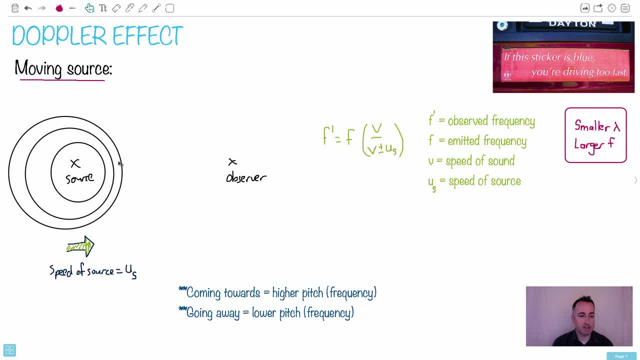 you look here these, do you see these little differences right here? These are actually the difference in the wave fronts. So you could actually define this distance right here. You could say that's lambda. So is this? Now compare that lambda to this one over here. Look this lambda here. I mean, I didn't draw it perfectly. 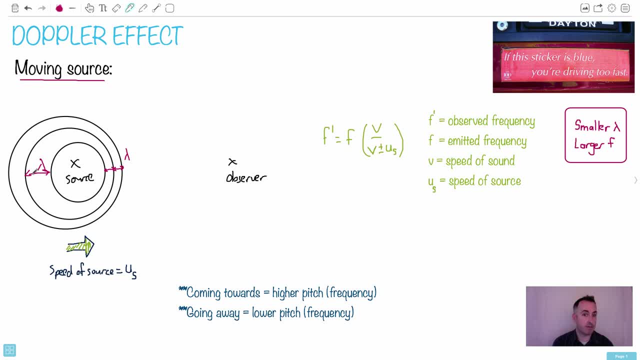 These should be even spacing here. But do you notice this lambda over here is smaller than that one. So here's a little trick for you: When you have lambda is smaller, that means you have a larger F. That's because lambda the wavelength and 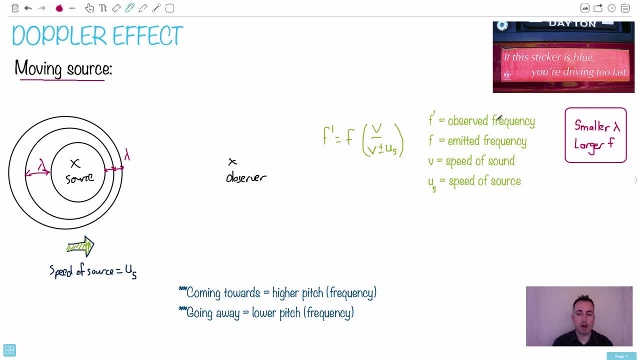 the frequency work in opposite directions. If you forgot that, you can use the wave equation: V equals F- lambda, You know that's the speed of the wave and this is the frequency and the wavelength. So if you wanted to do this, can you see if V over here was going to be the same If lambda gets smaller and then F? 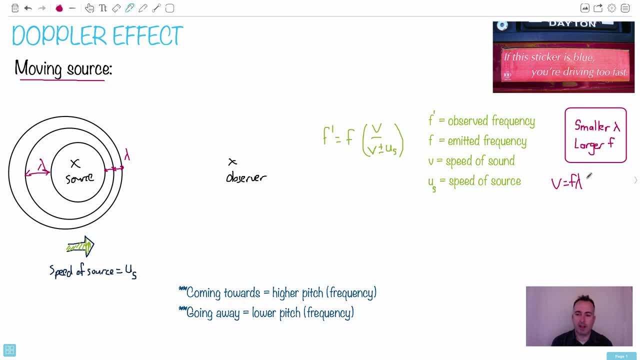 has to get bigger. So this equation is sort of helpful in order to sort of figure out what happens here. So if lambda goes down, the frequency has to go up, Where they work in opposite directions in that sense. So what this then means. think about this. If you're observing this sound here, this is a. 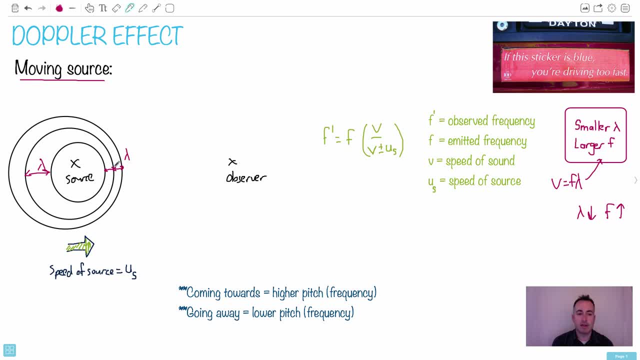 sound coming towards you, Well, the wavelength of the sound is smaller. Doesn't that mean then, the frequency is larger if it's coming towards you? So that means, here, as it comes towards you, you're gonna hear a higher frequency. as it comes towards you And, of course, as it passes by you. Can you imagine now this? 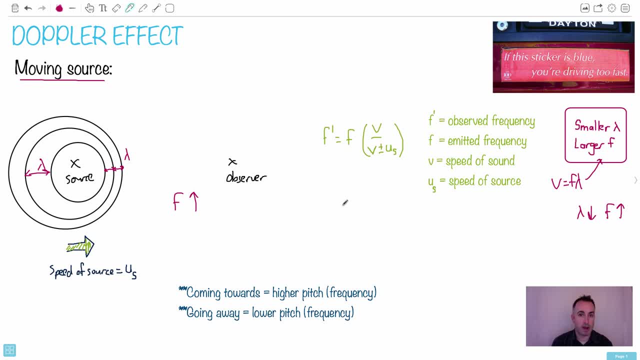 whole thing right here, Being sort of over here now, Can you imagine it being to the right? Do you notice that then you'd have larger wavelengths. So if you had larger wavelengths that means you'd have smaller frequency, And the frequency really kind of tells you what we call the pitch of a sound. So you know if 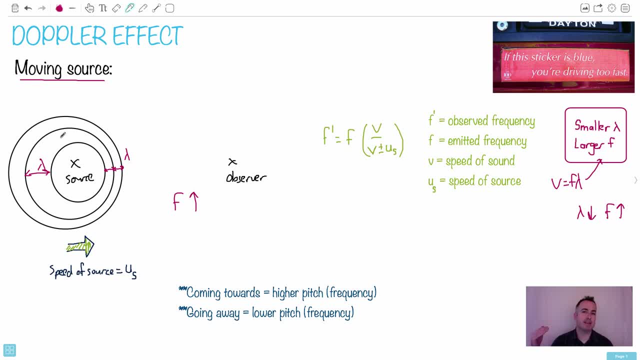 something has a higher frequency. it's like you know, like you might have seen, this with car racing, As a car passes by the camera, for example, you know if you see, if you're stationary observer and there's a car coming past you, it kind of 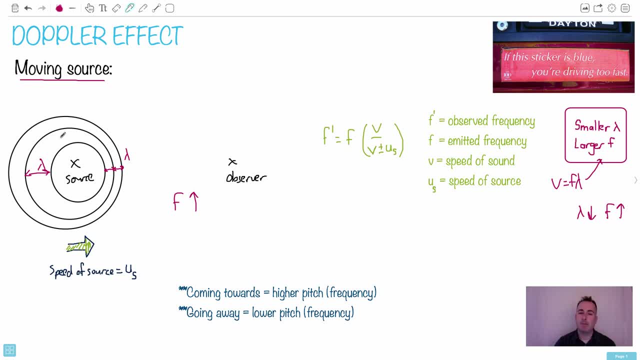 goes like this. Why does it do that? Because, as it's coming towards you, the frequency is higher. That's why it's like. I know I sound like an idiot when I do it, but that's fine As it goes and as it passes in front of you, of course. then it's 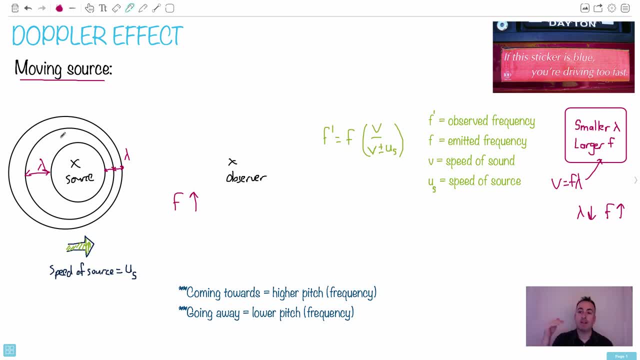 going away from you. So larger wavelength, lower frequency. That's why the sound seems to go down in pitch. Keep in mind that's sort of how it works. I know I'm sounding like a moron when I do it, but there you go. 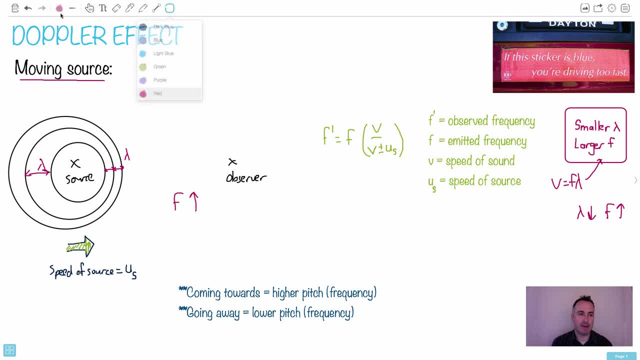 So this right here is the Doppler effect equation. This is the main one right here that you need. We're gonna talk about this because you're gonna have observed frequencies and emitted frequencies, So this is why it's really important to then break down this equation here. So F' is gonna be. 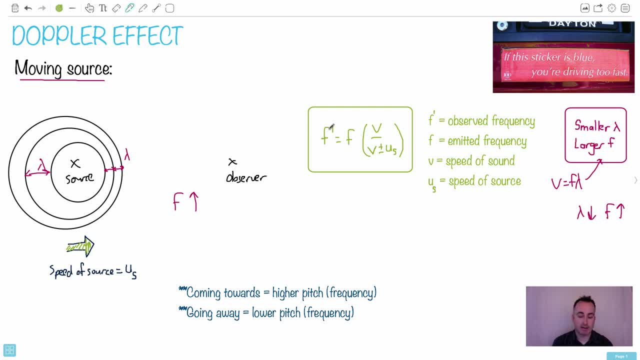 the observed frequency. That's what you, the observer, actually detect. It's gonna be equal to F, which is the emitted frequency. That's what it's actually putting out, You know, if it's like honking its horn, for example. 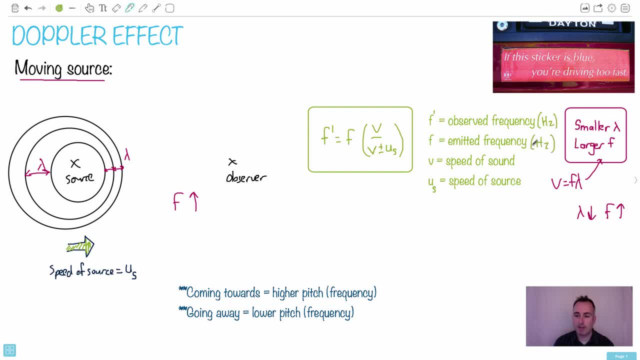 By the way, frequencies, those are measured in Hertz, aren't they? or in one over seconds. this v and this v are the same v, that's the speed of sound, which is in meters per second. so if it's an air it should be, like i don't know, 330 ish meters per second. and then us here, this. 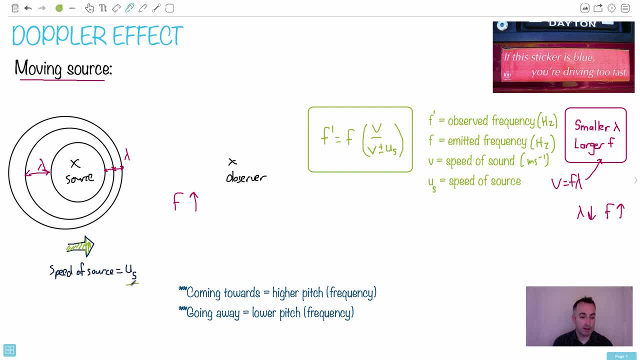 is the speed of the source, that's how fast the source is actually moving. this is also in meters per second, so it tells you basically, the faster your source moves, you know, the more this shift should happen. now, when do you use the plus or the minus? there's some ways. i mean, you could, you could. 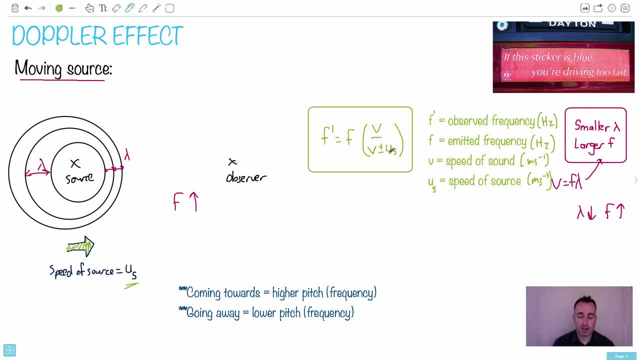 uh, you could actually try to calculate it. um, you could learn the different ways. but what i'd like to do is just think about very carefully. if this thing is coming towards you, you know the frequency should be higher. you know, if it's coming towards your, frequency should be higher. so which value of 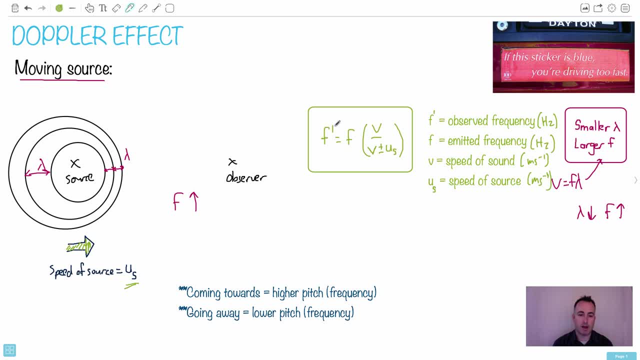 us plus or minus would make the frequency observed be higher, you know. so which one would make that f prime to be larger. so would a smaller value on the bottom see if i, if i did a smaller value on the bottom, that would make this value bigger. so that's how i sort of think about it. otherwise, 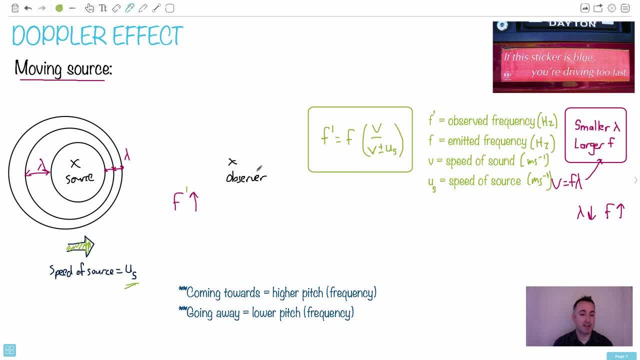 you can always just try to do both calculations and whichever one gives you the larger frequency. you know, if it was coming towards you, then you do that, because if it's going away from you it'll be the opposite side, i guess. then the frequency should be lower. i just think about cars coming. 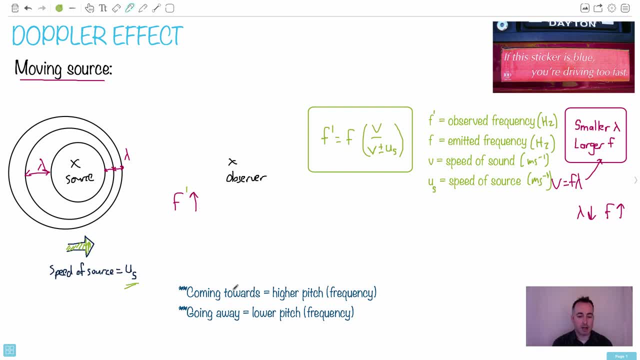 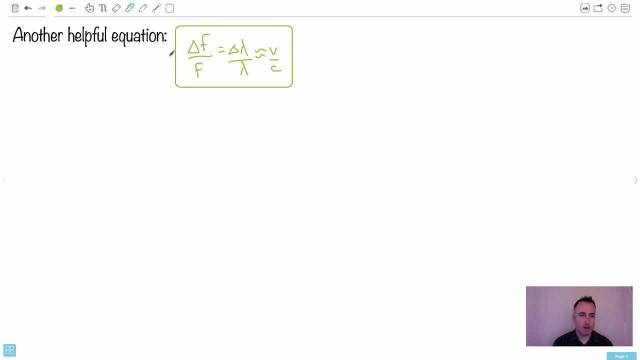 towards me and that tells me if you should go up or down. so that's why i said: coming towards you is higher pitch or frequency, going away is lower pitch or frequency. so let's, uh, look at this. we have another helpful equation. this i'm not going to say much about because it's on your data booklet, but 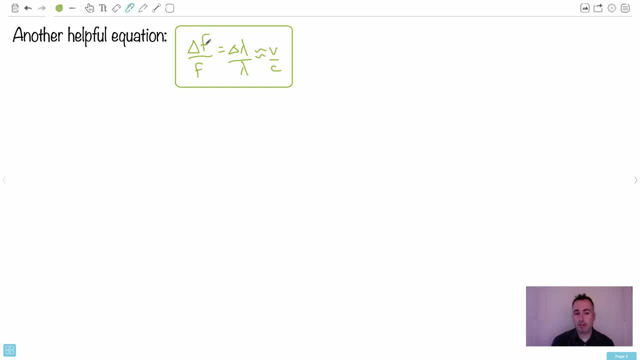 it just tells you: um, a change in frequency over the emitted frequency is equal to change in wavelength over wavelength, which is related to v over c. this is helpful for astronomy, for example. if we see, we observe something's wavelength being different, then can you see that we. 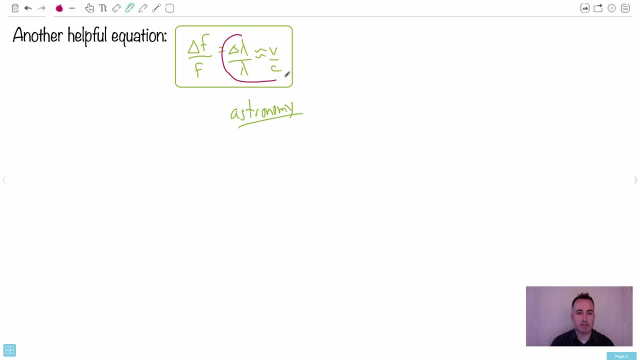 can actually infer its speed as a fraction of c. so you see this one here, do you see? uh, this see, remember the speed of light. so we can actually say then that, um, you know, if we see the wavelength of what we're seeing in a star, let's say we see some, uh, some emission lines or some absorption. 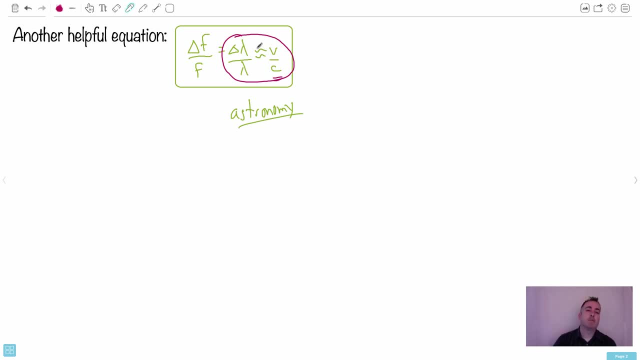 lines or something, uh, that we're looking out into space and we see something. and we see those lines. they're shifted a little bit, either blue or red. right, this is the whole idea about red or blue shift. we say things are shifted because if they're shifted to larger wavelengths, uh, that means they. 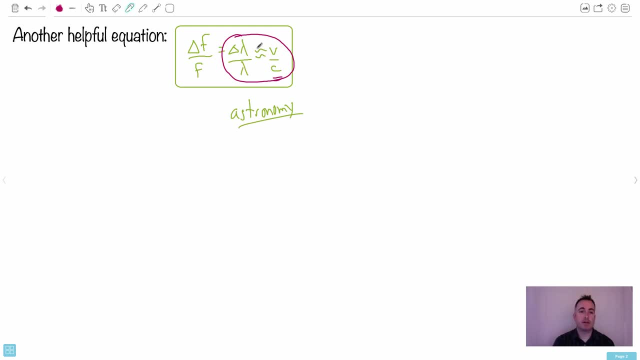 get more red, and red shift it means you know things are going away from you, and blue shifted means they're coming towards you. it turns out almost all the objects we're looking at are the we look at in space. they're pretty much all redshifted. In other words, everything is. 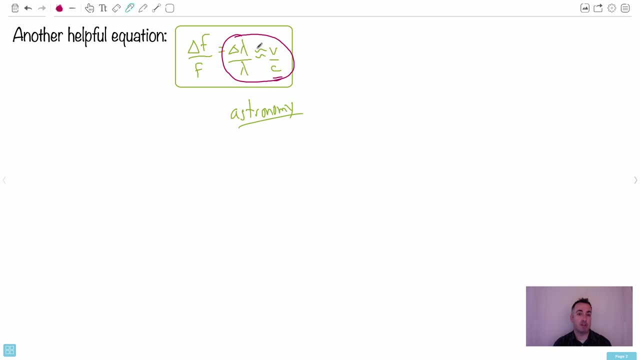 going away from us. This shift, this amount that's been shifted by wavelength, that's this delta lambda. From there, you can see, you can figure out your speed as a function of c, as a fraction of c. I mean. Here's an example: Here you're driving your car at 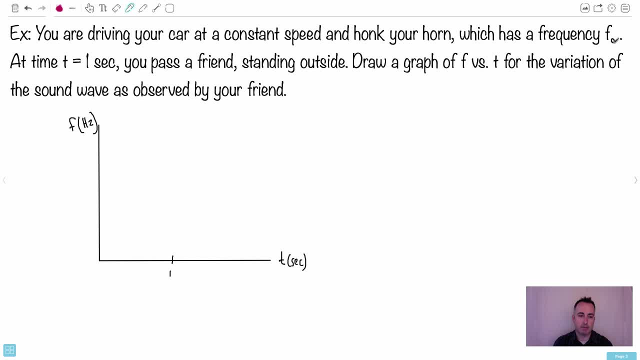 a constant speed and you honk your horn, which has a frequency f0.. We're going to assume that we have some sort of frequency f0 here Now. at time t equals one second. what are you going to do here? You're going to pass a friend who's standing outside. Imagine then. 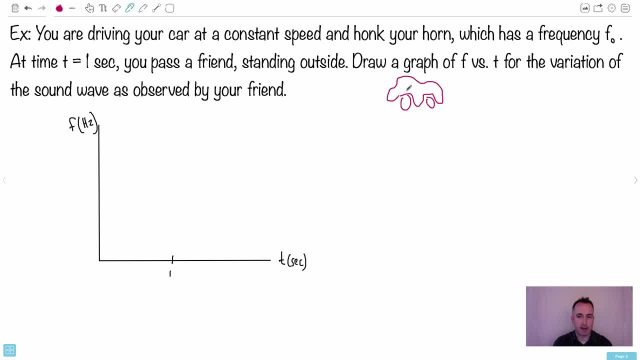 you're driving your car here like this. Oh boy, that is a bad car. This is me in my car. I'm not an artist, you can tell. This is me driving towards my friend here. He's sad because he thinks I'm going to crash into him, maybe because clearly I'm not a very good driver. 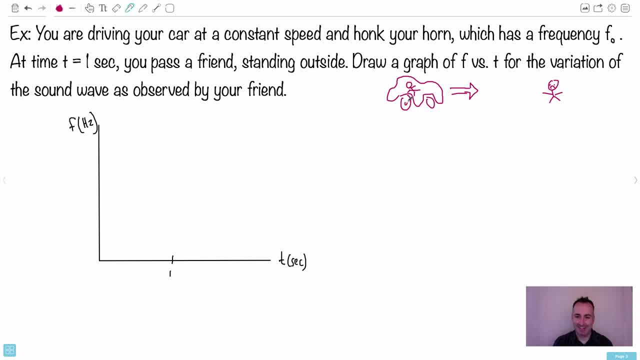 if I'm not even driving in the car, I'm sort of outside it. I don't know what's going on here. So this is me honking my horn right, So my horn sound is coming towards it. So what's happening then? Remember, draw a. 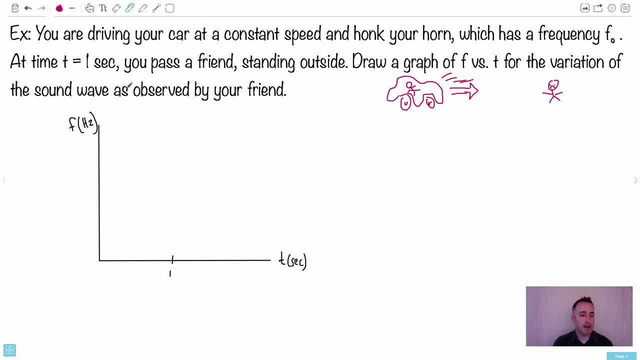 graph of F versus T for the variation of the sound wave. So what's going to happen is this: I'm going to be: well, let's assume we have some sort of constant value. This is what he, or this is what my actual sound is, which is F zero. let's just say- And at this point this is the important- 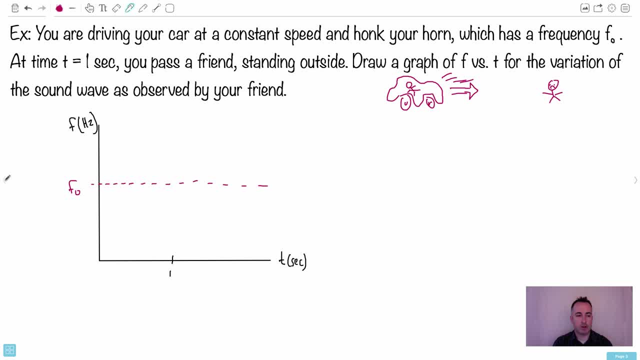 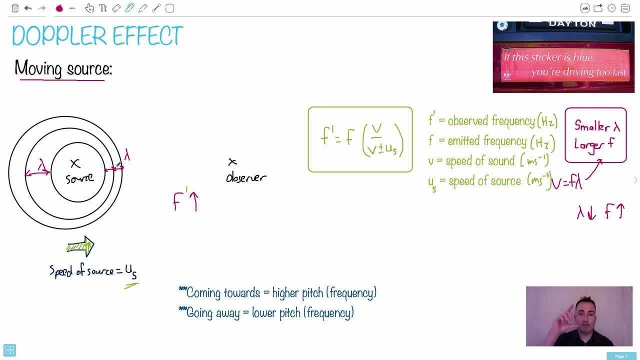 thing I pass, my friend, Remember what happens as I'm coming towards like moving a source, as I'm coming towards higher pitch or frequency. Remember that's because the wavelength got squished. And remember, if wavelength goes down, frequency goes up. That's why I think of it as I.